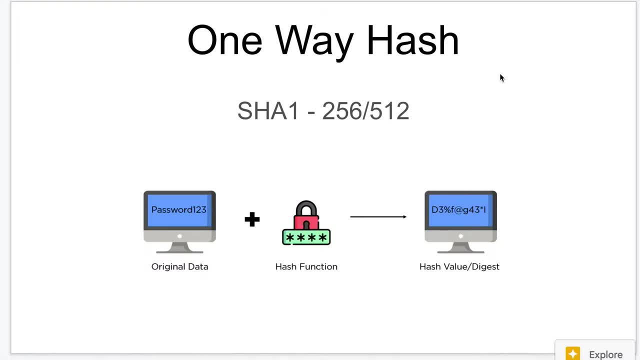 Hello and welcome. In this video I want to go over what is a one-way hash. They're very popular in computer science for securing data, encrypting things of value, and so I want to be able to describe that to you. So in this video I'm going to go over what that is, and then in the next, 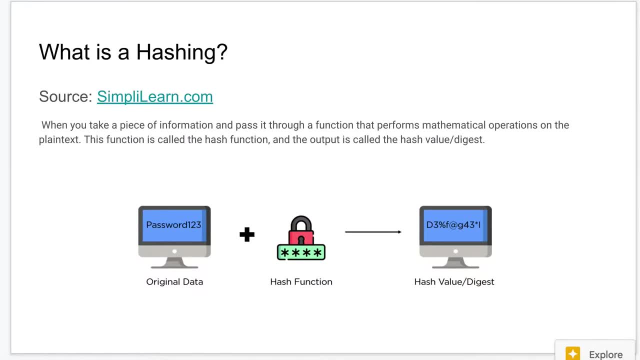 video I'm going to go over how we can program it using Java. So what is hashing and one-way hashes? It's basically when you take a piece of information that could be anything like a password or like a large document and you pass it through a function that performs mathematical. 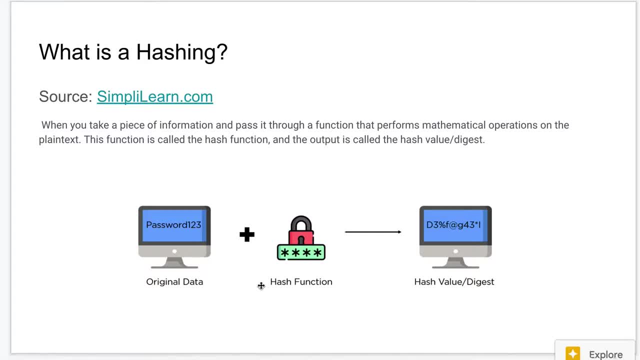 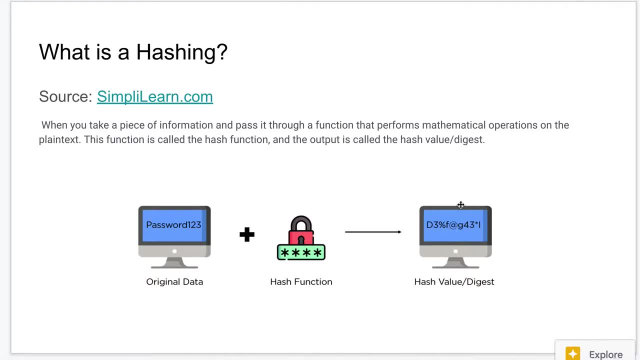 for all intents and purposes, is the one defining. characteristic of the one-way hash is the mathematical equation that happens here, that produces this is not meant to. there doesn't exist a algorithm to reverse it, So that's why it's one way And that's what makes it very secure. 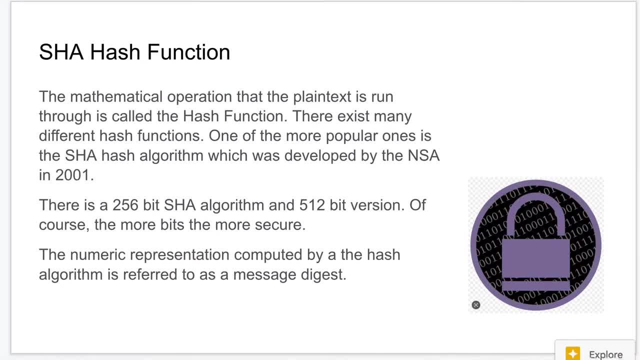 And they're widely used. This, the one that I'm talking about, I'm going to mention here, and then we will program using Java. It is called SHA, which stands for secure hash algorithm, And, as you can see here, it says it was. 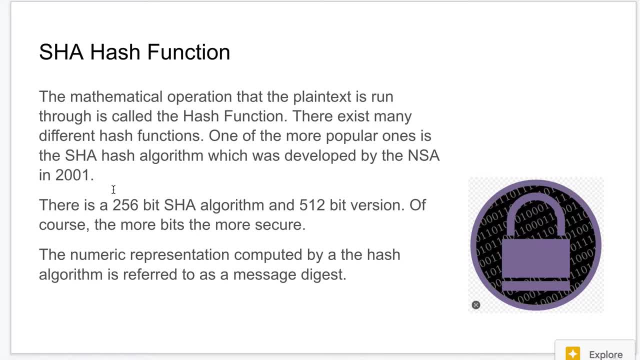 developed by NASA in 2001.. That was SHA-1.. And there's since been a bunch of variations of it, including SHA-256 and 512.. And, as you might suspect, the more bits the more secure it is. And yeah, and so there's actually even an SHA-3,, which is a higher end version of the 512. 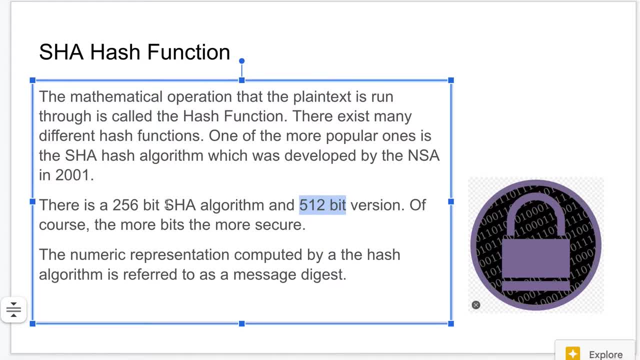 And these are still. SHA-1 and SHA-256 are not recommended anymore, but SHA-3 and, I think, 512 are still kind of widely used and sometimes now just incorporated into other algorithms. So yeah, I there's, there's some good articles. there's some good articles, there's some good. 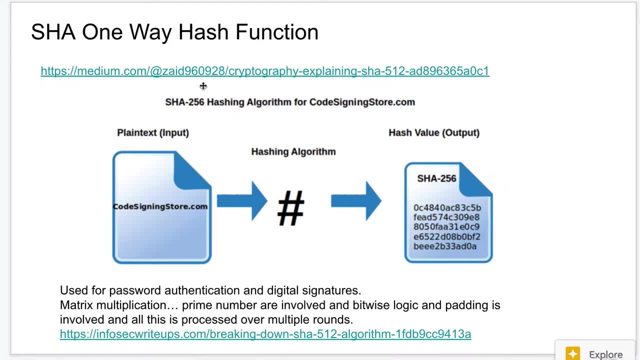 articles that I'm linking in the description here. If you really want to try to understand the math, I will just say I don't really understand the full algorithm as far as the math is concerned. I do know that there's some matrix multiplication going on for, basically, 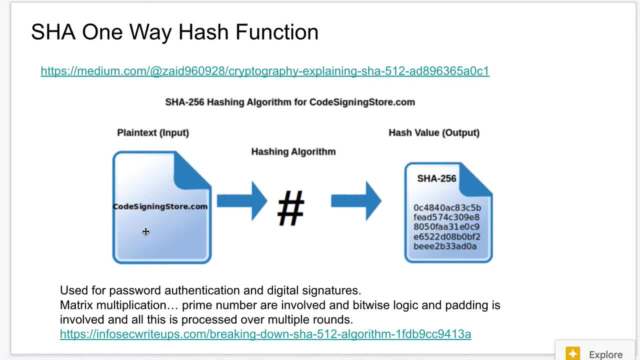 when you input something, for chunks of that something are multiplied against some prime numbers, And there's also some bitwise logic involved- XOR type stuff- And I know that those chunks of data are padded if needed. And this this process happens over multiple rounds, so that it's starting to sound very complicated, And that's what it becomes. 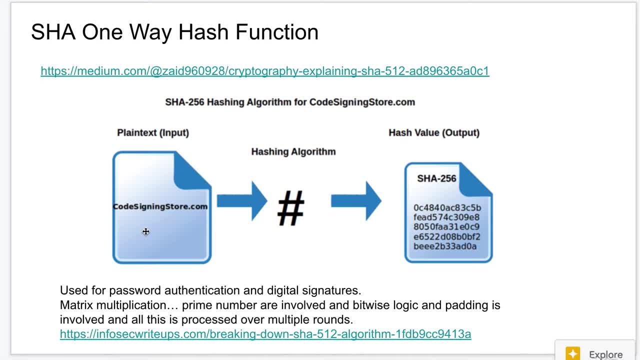 this complicated value, hash value That is. if you do this, this part in here right should be very difficult to figure out what this represents. It's used commonly for password authentication and for digital signatures, And so how it's used in that capacity is you put in your password. the hash algorithm is performed. 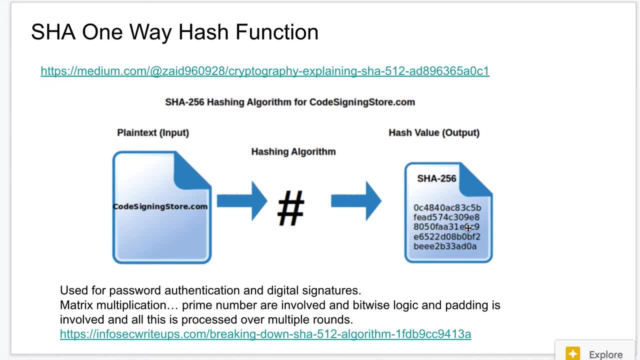 and then the hash value is actually stored. Let's say this was for a website, it would be stored on that web server, right? And that's great, because if somebody hacks that web server, they don't get access to your actual password, They don't get access to your actual password, They don't get access to your actual. 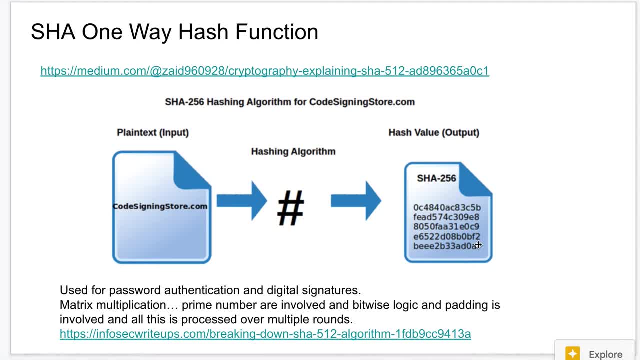 password. They get this hash value, which you know, the the more modern hash algorithms. it is very hard to figure out what this represents, if not darn near impossible. And same same goes for digital signatures. You can send a document to someone. 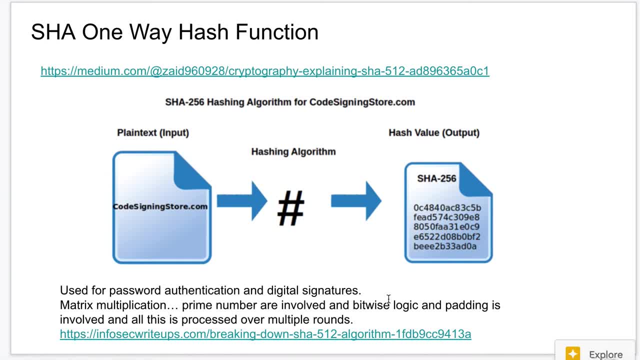 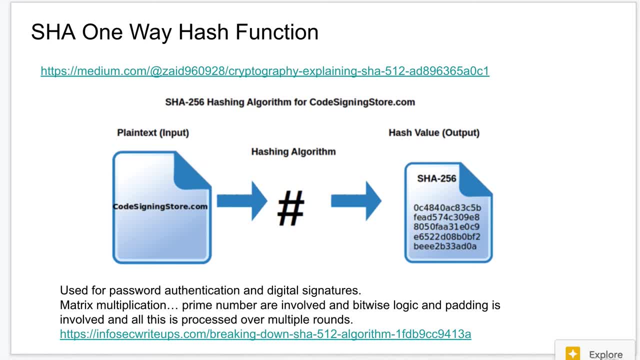 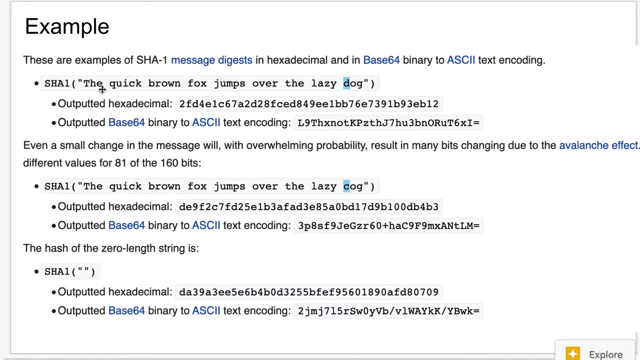 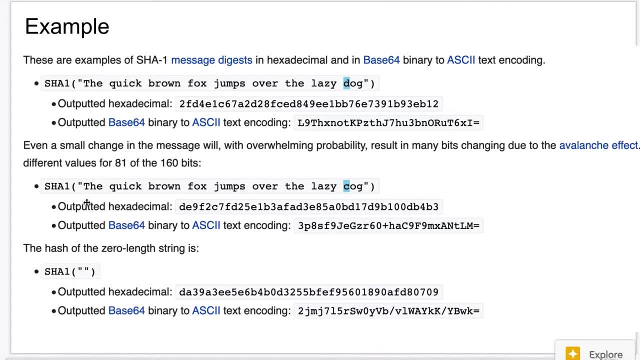 The quick brown box jumps over to lazy dog. And then the second example: here it's: one letter has changed from dog to cog and the whole output here is totally different, which is a great feature of this, And that's what makes it so important. And that's what makes it so important, And that's what 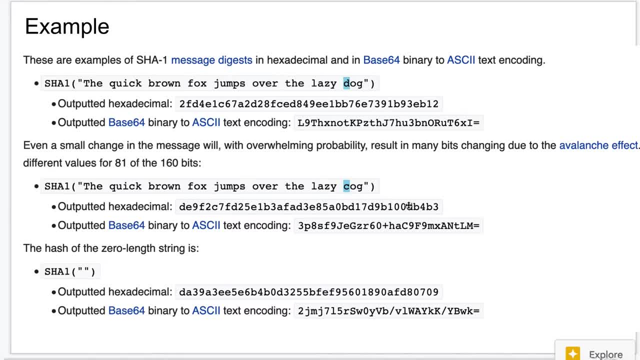 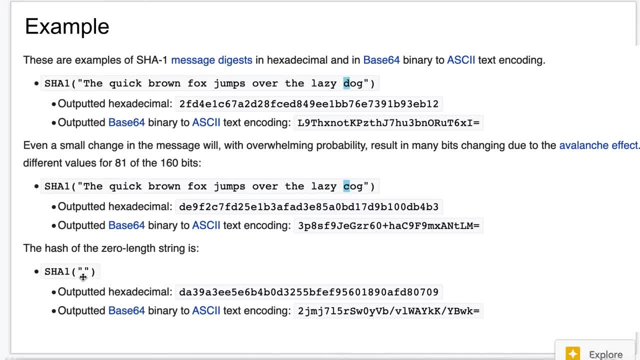 right, And, as you see here, this is kind of cool too. You can literally just put in one character and your output would be something like this: And this is the SHA-1 where the I have a link in in a I'll show you in a second to a future slide where you can actually play around with, I think. 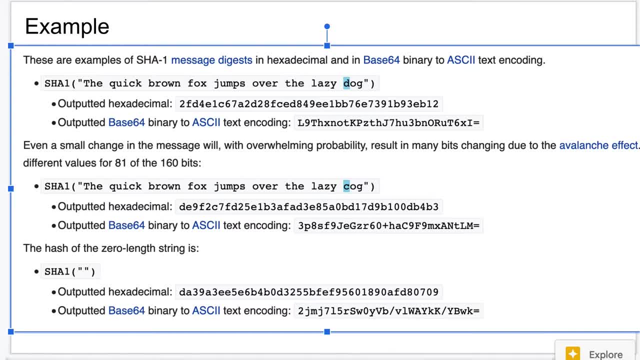 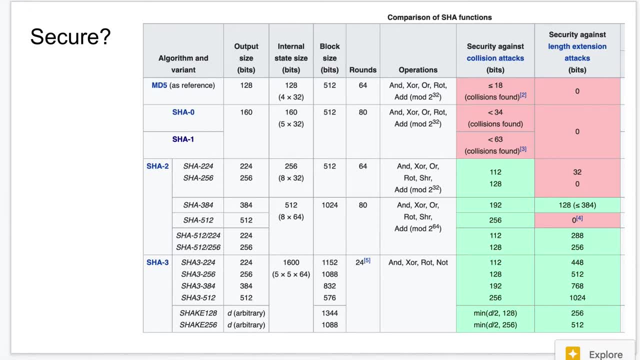 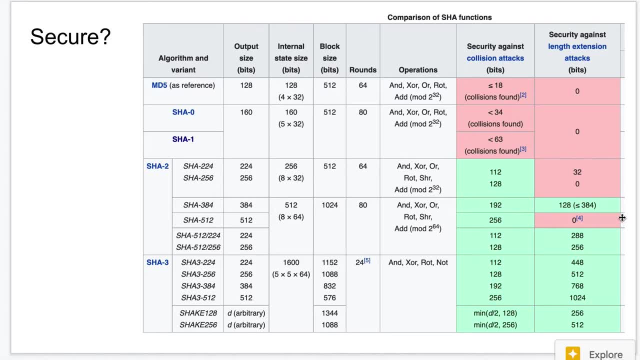 and one, and some of the twos are not recommended anymore because they've been compromised. People have figured out how to kind of launch attacks against them And there's different collision attacks you can do, which is really cool, And that's what makes it so important. 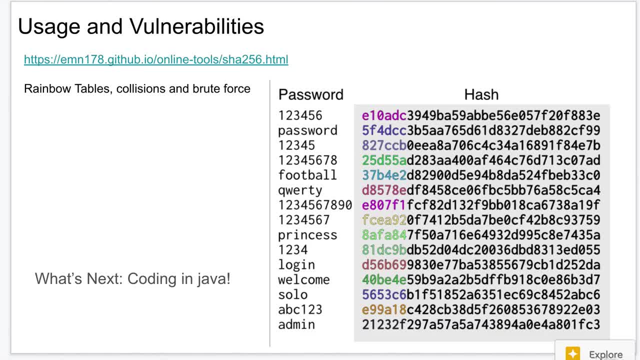 Which basically means I'll show you an example Like there's. all these hackers will try to do things like create rainbow tables, where they could. they figure out that this is a common password. So when they they hack a web server, they were able to figure out that this common password results in this, And so they could. 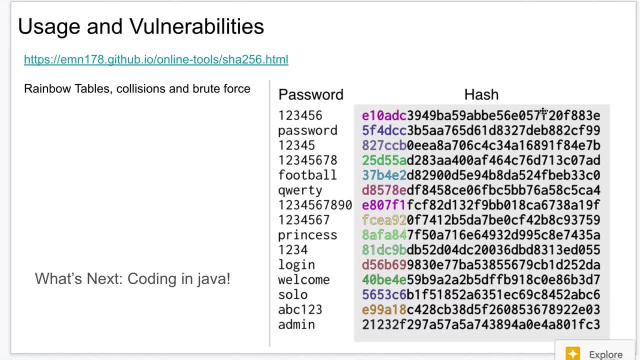 use that to. I mean honestly, if you use a password that is fairly unique, you shouldn't have to worry about this. But if somebody uses these, don't ever use these. but if somebody uses these passwords that you see here, hackers have these rainbow tables. 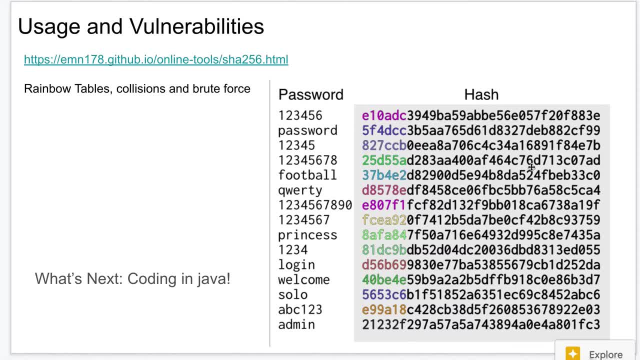 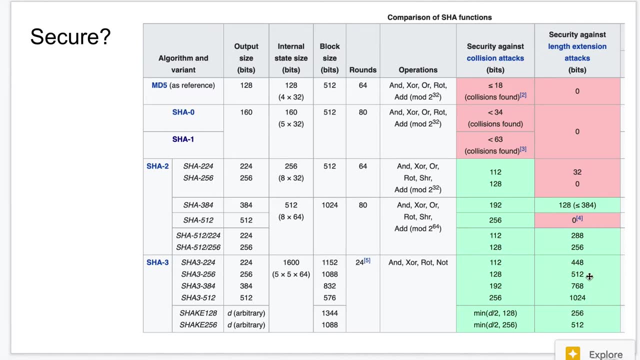 what they're called that. can they can figure out what the hash output would be for that? Yeah, And then there's some brute force that you could do. but, like I said, the good luck. brute forcing some of the more modern versions- that it's just really tough, I'm sure. 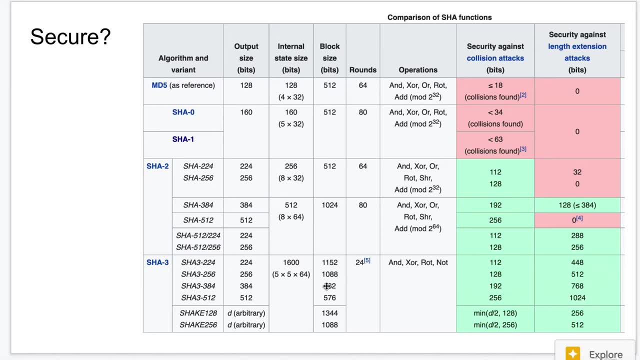 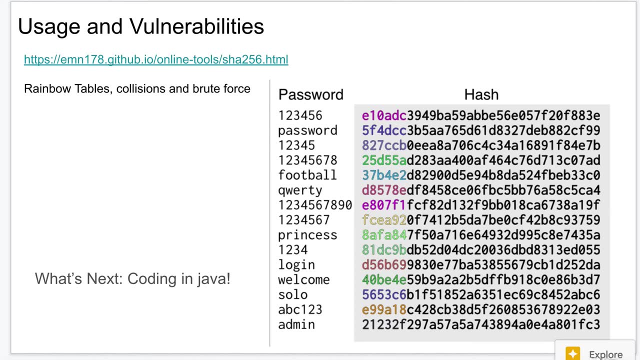 as computers get faster, hackers will figure that out, But right now these all look to be really strong- the ones I'm in green here, So you shouldn't have to worry too much about that. So, yeah, that that's. Oh, I mentioned collisions here. Collisions are. 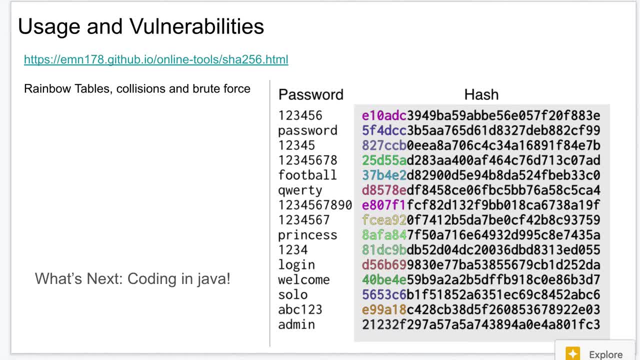 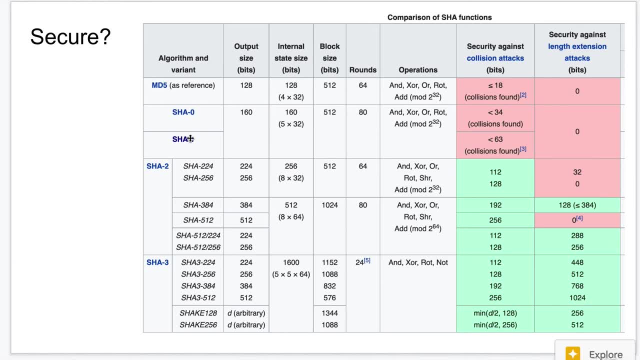 if you put in two different inputs and they produce the same output. that should never happen. It has happened, I guess, for some of the earlier ones, But you know the if you're, if you're the modern ones, that shouldn't be a problem. 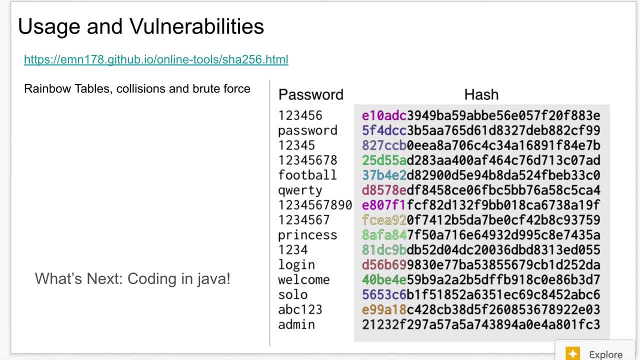 And so yeah, so that's it. I think I've covered everything that you would want to know about one-way hash and hashing, and the next video, like I said, I'm going to talk about how we can code this. It's actually not that difficult with some of the Java's built-in libraries, So yeah. 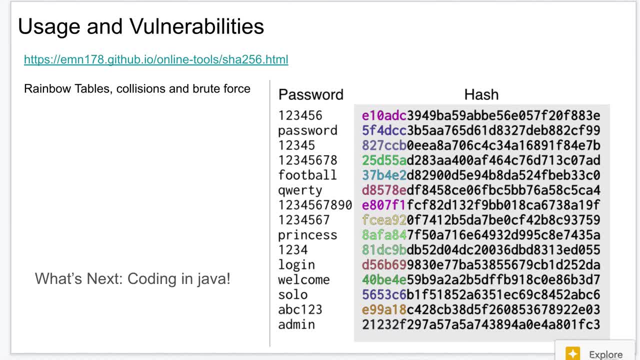 let me know. if you have any questions, though I'd love to hear from you, Thanks. 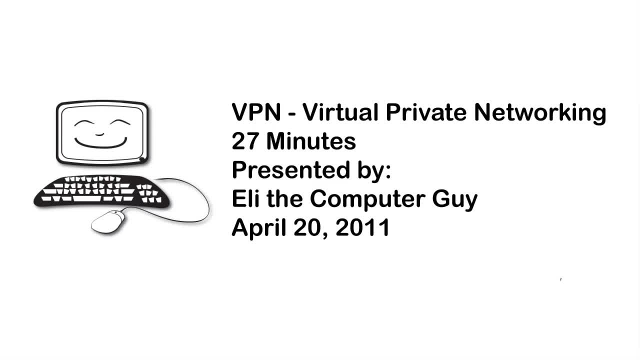 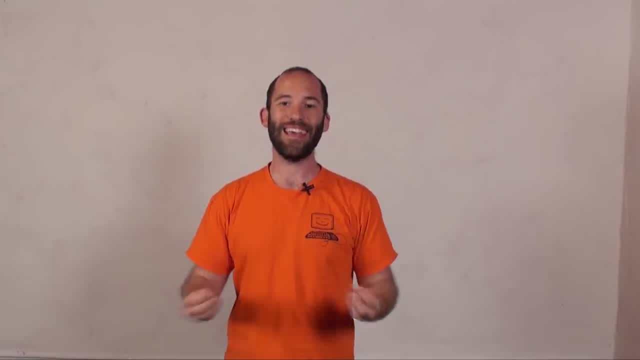 Hello again. as you know, I'm Eli the Computer Guy over here for EverymanITcom, and today's class is on VPN or Virtual Private Networking. VPN allows computers or entire networks to connect to each other over the internet securely. So if you have an office in Seattle and it. 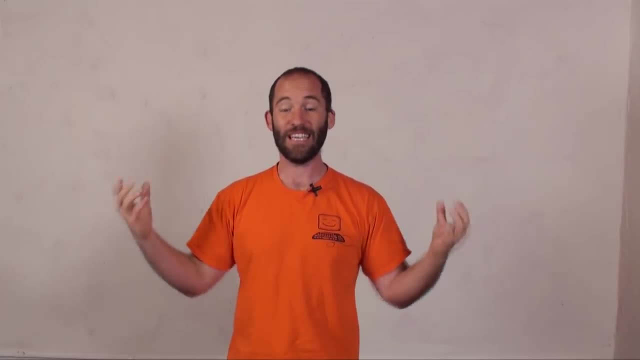 needs to connect to an office in Washington DC securely, you would use a VPN. VPN is a client server architecture, so you have VPN servers and VPN clients, and the software allows the VPN clients to securely connect to the VPN servers. Today's class is going to talk.